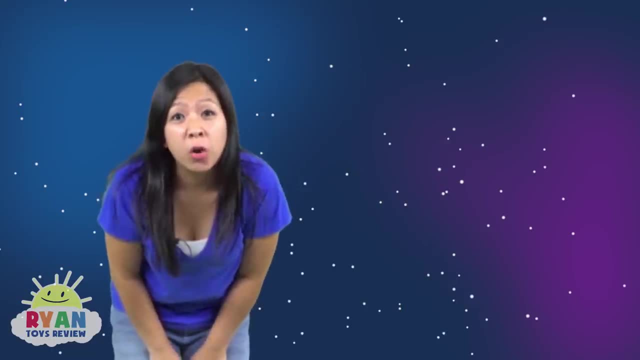 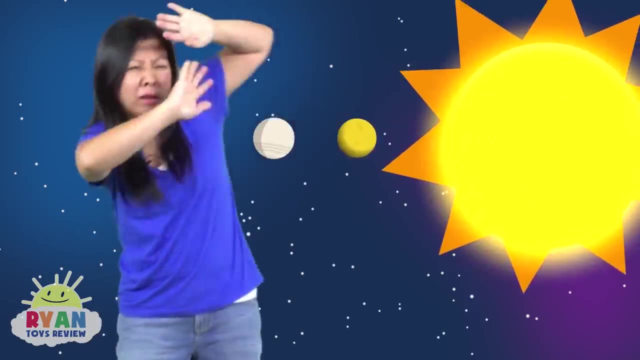 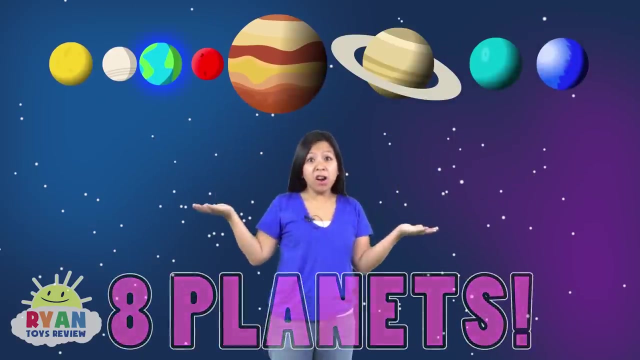 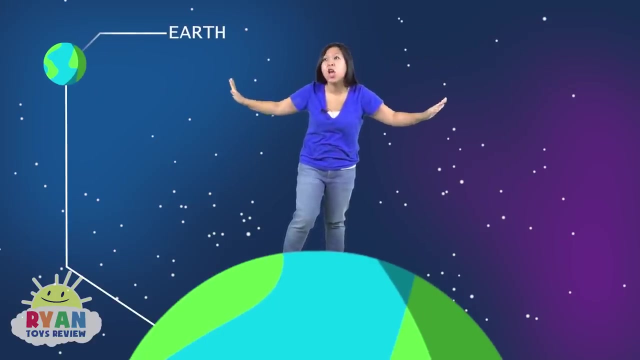 Whoa, Oh hi there. Did you know that Earth, the planet that we're living on, is the third planet from the sun. Whoa, the sun is hot today. There are eight planet total in our solar system, and Earth, the one we're on right now, is the only planet known so far to have life on it. 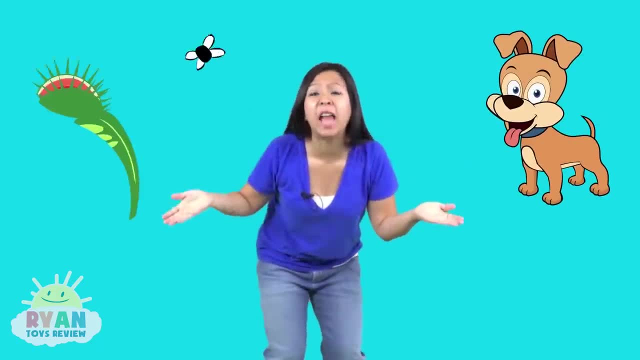 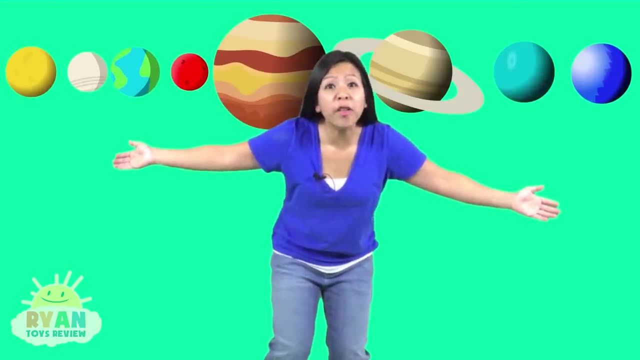 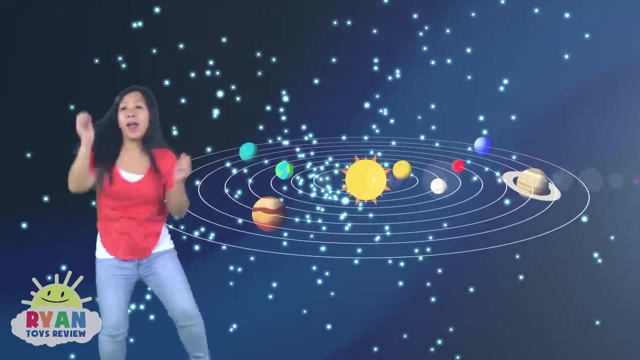 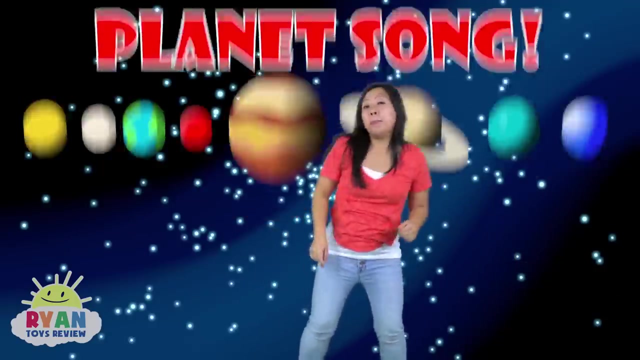 You can't find a dog or a Venus flytrap or human like us anywhere else. yet How cool is that? Let's learn all the planets' names and what they're known for. Are you ready? Let's go. This is the planet song. If you know the order, sing along. Planets revolve around the sun. 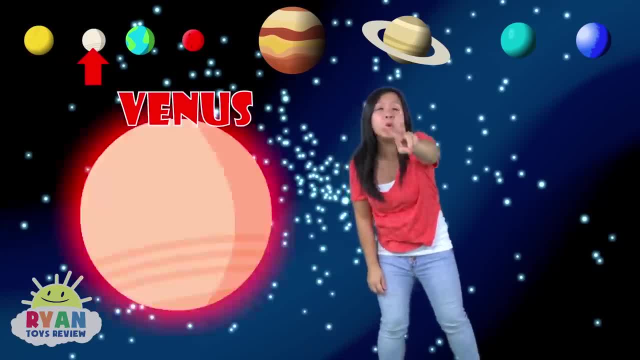 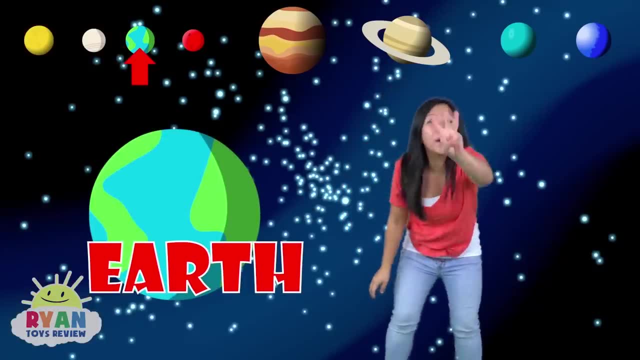 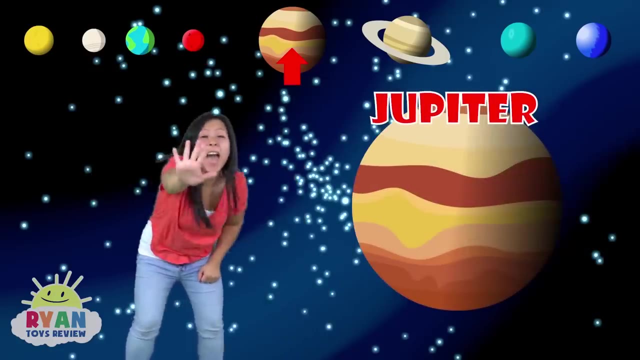 Mercury is number one. Venus is number two- It's too hot for me and you. Earth is the place to be. It's planet number three. Now let's learn some more. Mars is red and it's number four. Jupiter is number five and it's known for its giant size. 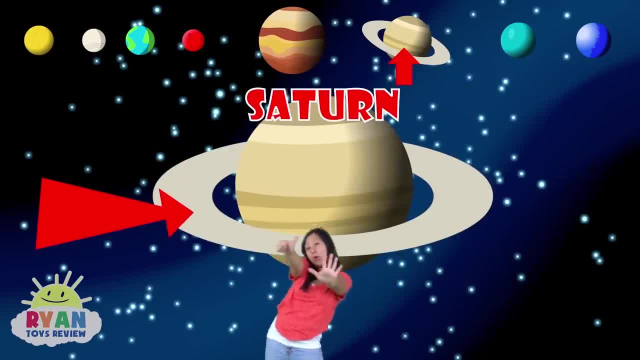 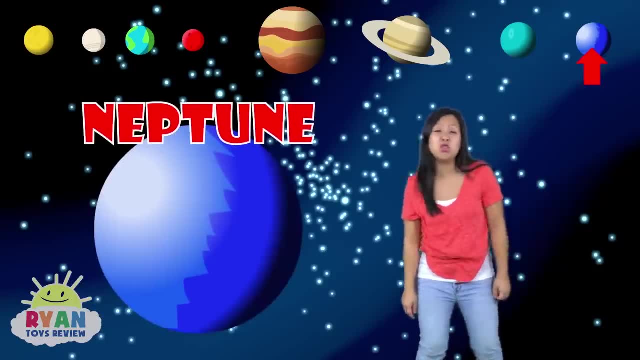 Saturn is the one with rings. It's number six in the order of things. Seven is the planet with ice, It's Uranus, and it's been on its side. Number eight's called Neptune, It's the last one and it's blue. 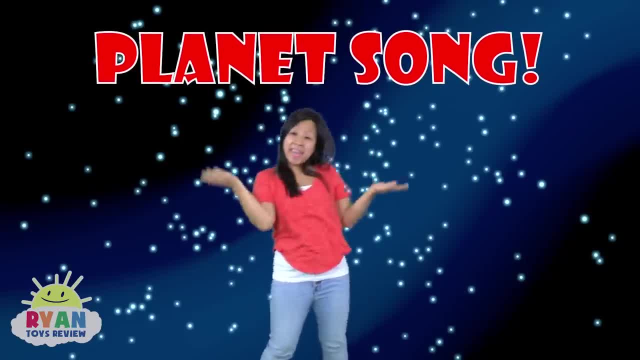 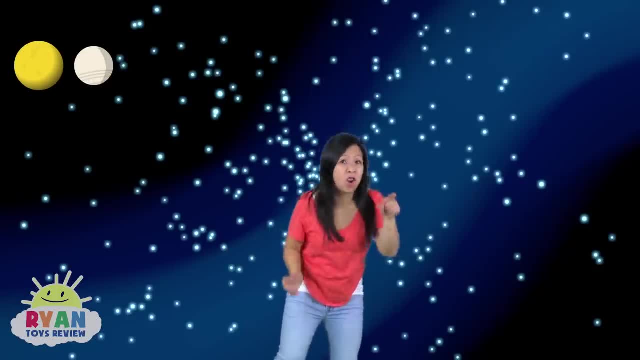 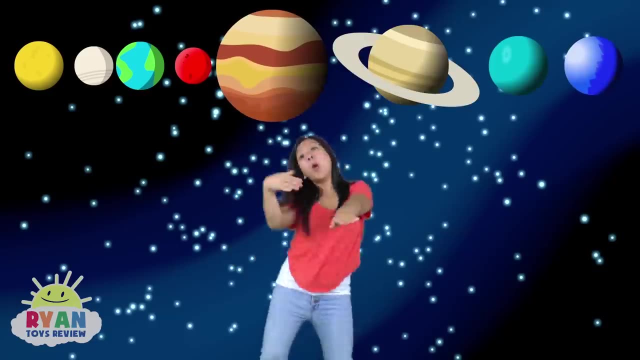 This is the planet song. Now you know the order. Sing along. Mercury, Venus, Earth, Mars, Jupiter, Saturn, Uranus and Neptune. Mercury, Venus, Earth, Mars. Mercury, Venus, Earth, Mars, Jupiter, Saturn, Uranus and Neptune. 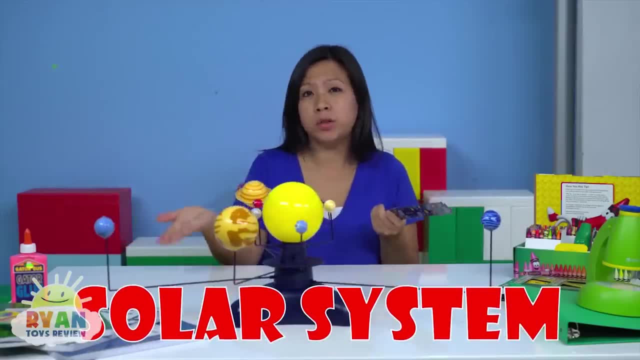 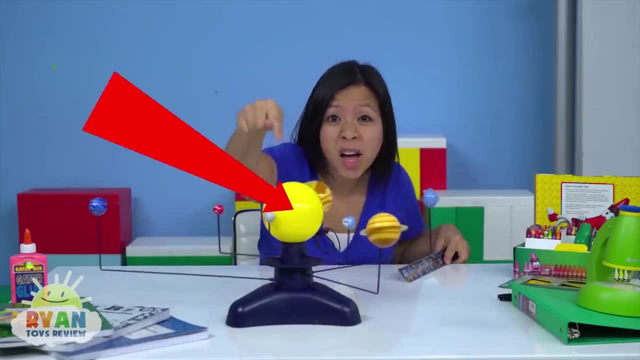 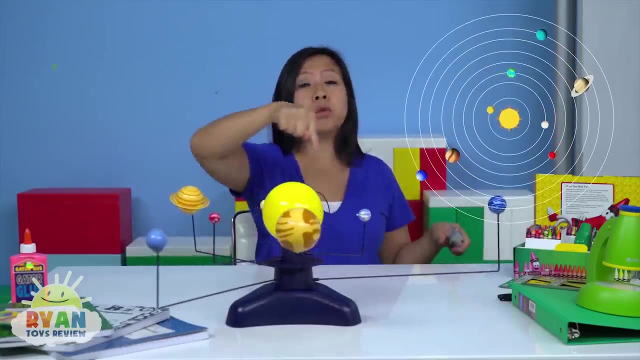 This is a very tiny model of our solar system. Did you know that all of the planets in our solar system revolves around the sun? That means that the sun right here is in the middle and all the planet goes around the sun. First we have Mercury. 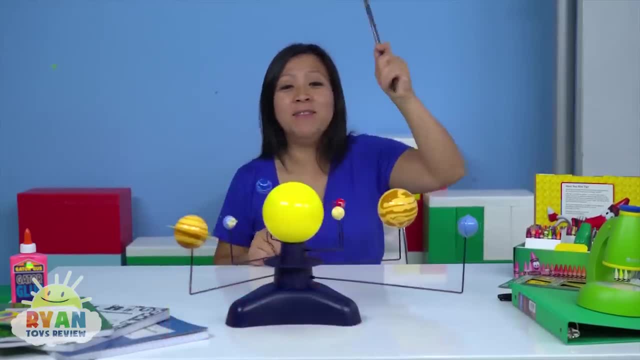 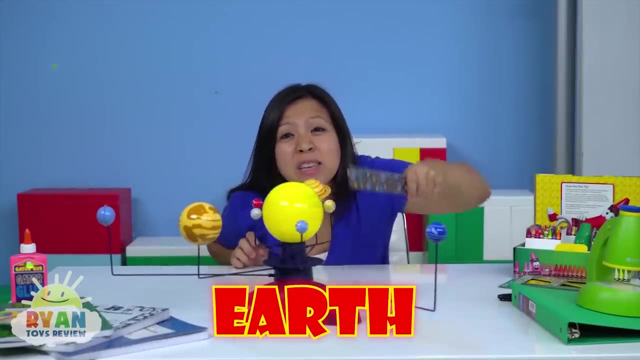 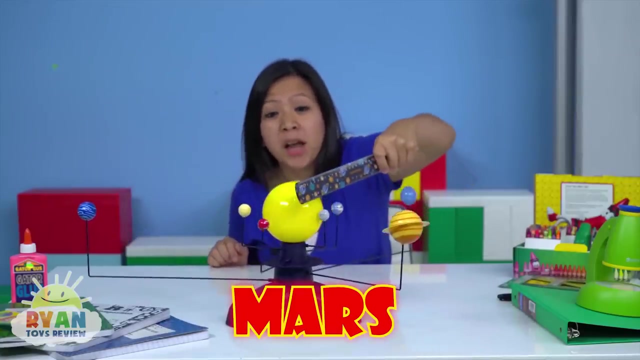 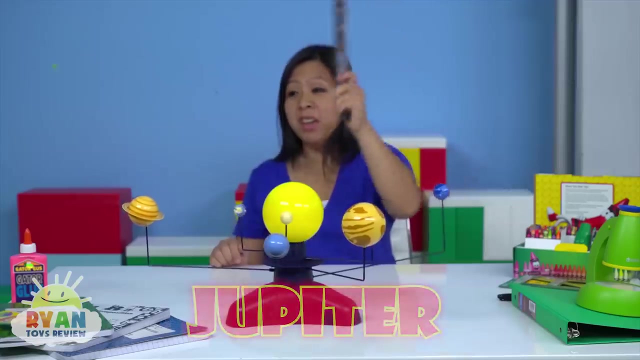 then Venus, then Earth, the planet that we live on, with the tiny moon there. I don't know if you can see. Here's Mars, which looks pretty red right. And then here is Jupiter. Look how big it looks. Then here's Saturn, with a whole bunch of rings around it. That's pretty neat. 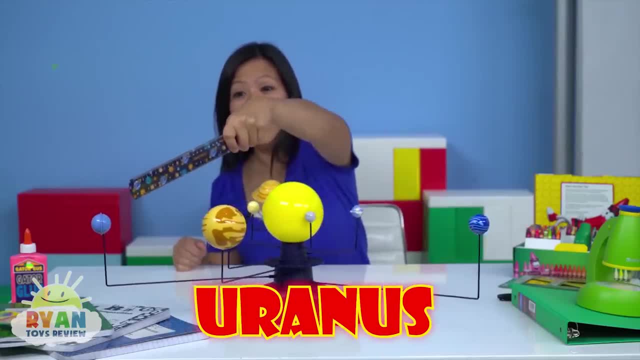 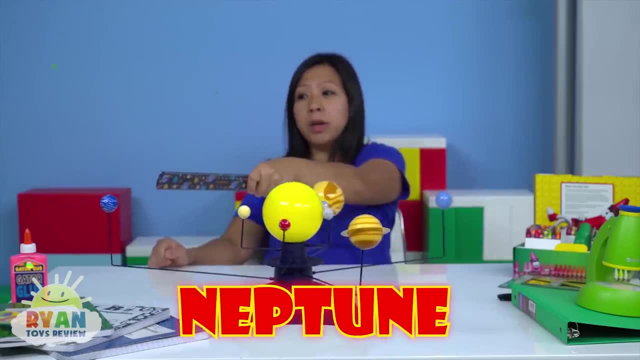 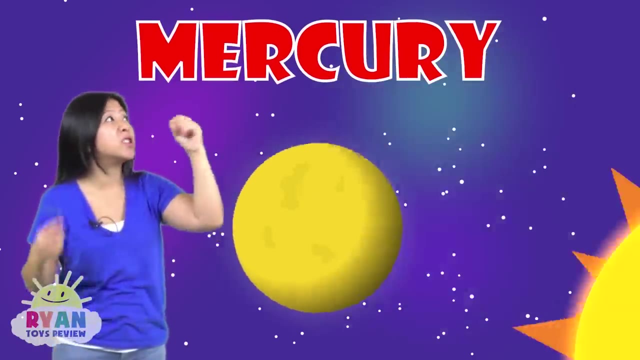 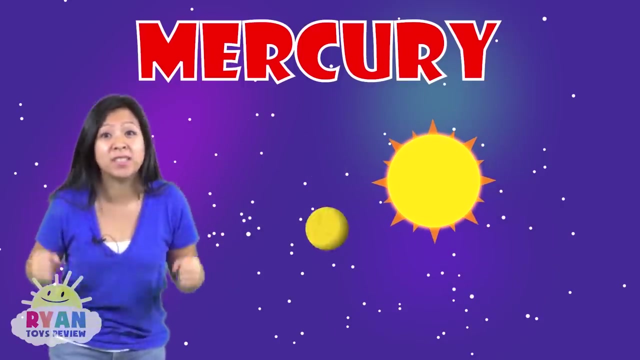 And here is Uranus. And then the ace planet, the furthest away from the sun: Neptune, right there- Look how blue it looks. This planet name is Mercury. It's the first one that is closest to the sun and it goes around the sun super fast, the fastest. 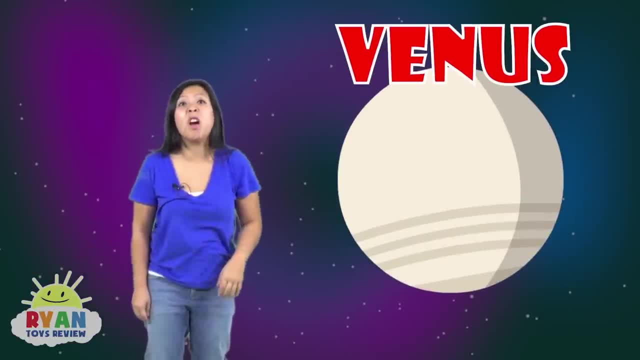 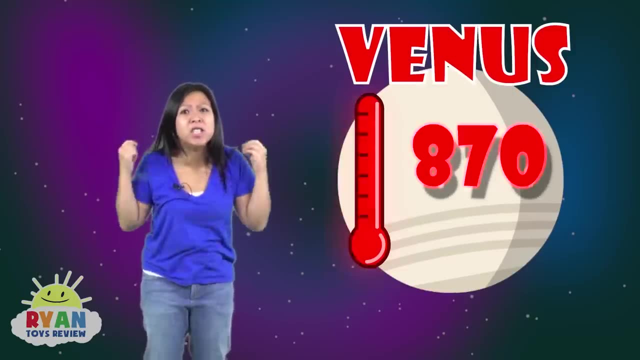 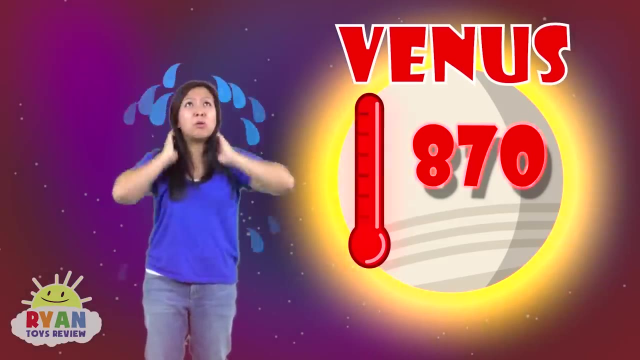 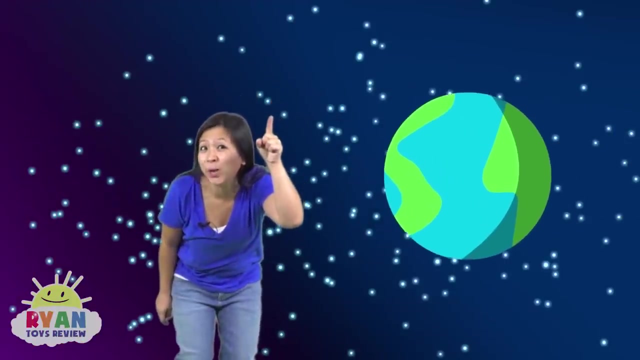 The second planet here is Venus. If you think Earth is hot, you wouldn't like Venus. It gets to 870 degrees. It is the hottest planet in our solar system. I'm sweating just being so close to it right now. And the third planet here is: do you know what this is? That's right, it's Earth, the planet that we're living on right now. Earth, the planet that we're living on right now. That's right. it's Earth, the planet that we're living on right now. Earth, the planet that we're living on right now. That's right, it's Earth, the planet that we're living on right now. 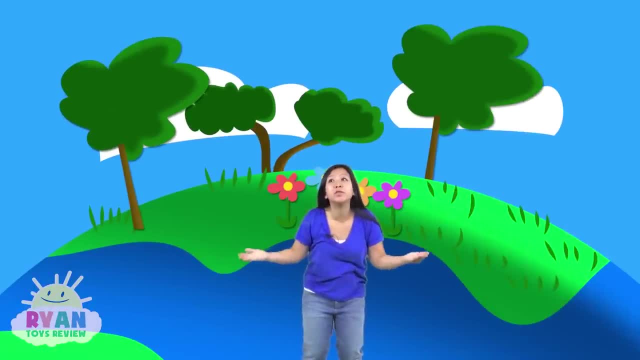 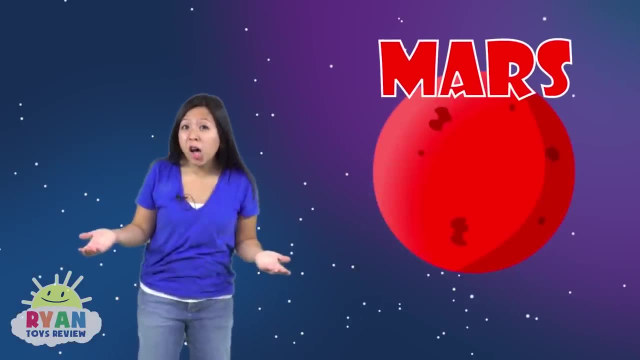 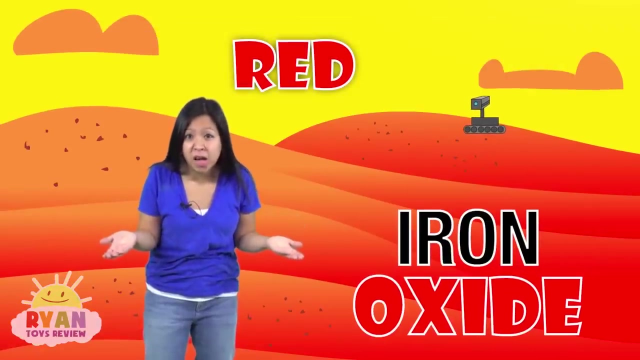 We're the only planet that we know of that has life so far. Pretty cool, right. This fourth planet here is called Mars, also known as the red planet. It's red because it has lots of iron oxide, which makes the soil look really red. 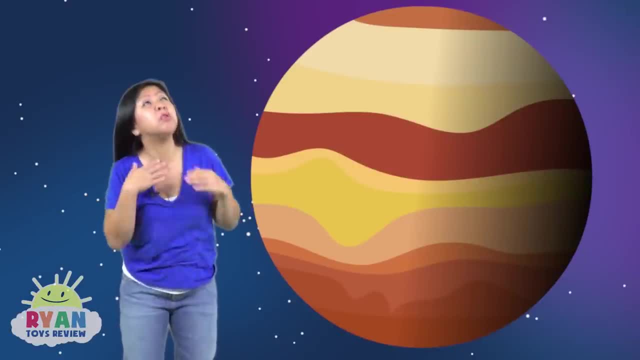 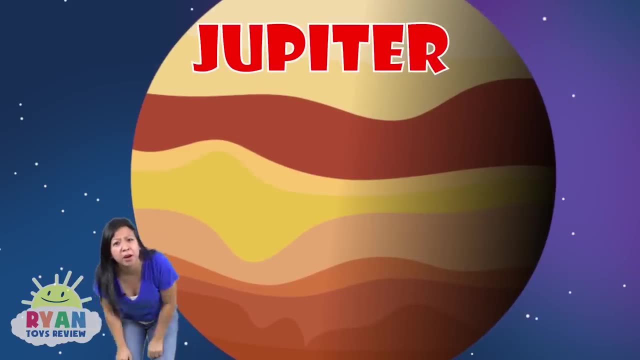 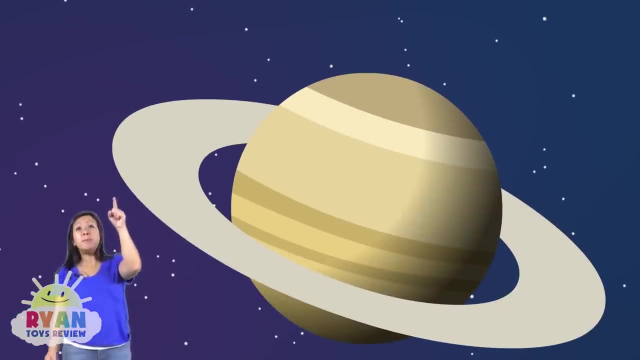 This planet here is the biggest planet in our solar system. It's so huge. Wow, Do you remember its name? That's right, it's Jupiter. It's 11 times bigger than Earth. And the sixth planet here in our solar system name is Saturn. It's known for its giant rings. 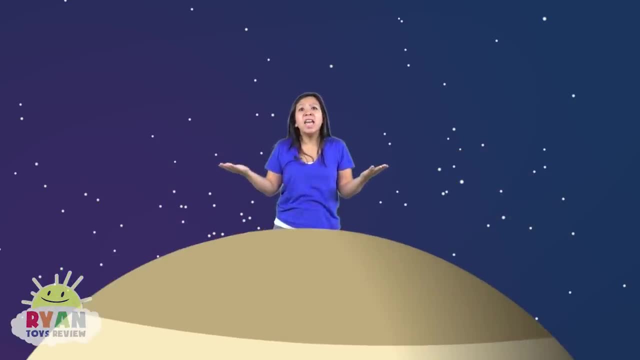 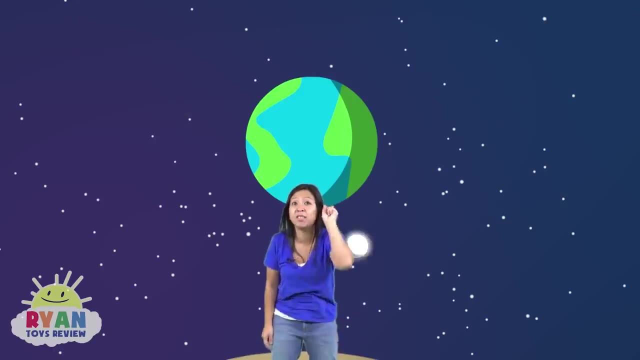 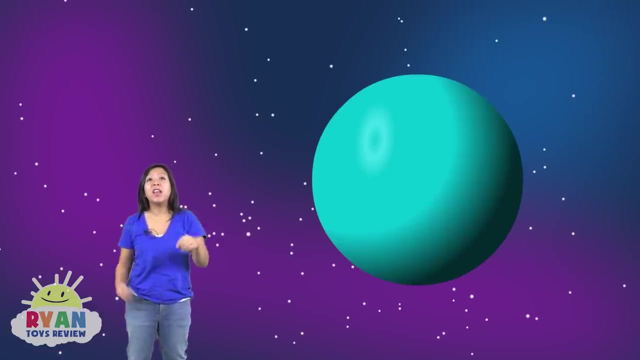 Not only does Saturn have rings, it has over 60 moons. Look, that's a lot of moons. Earth only has one moon. This next planet is super interesting. The seventh planet is Uranus. It spins. get this on its side. 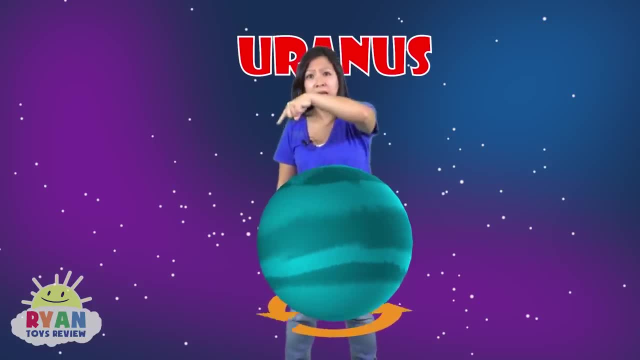 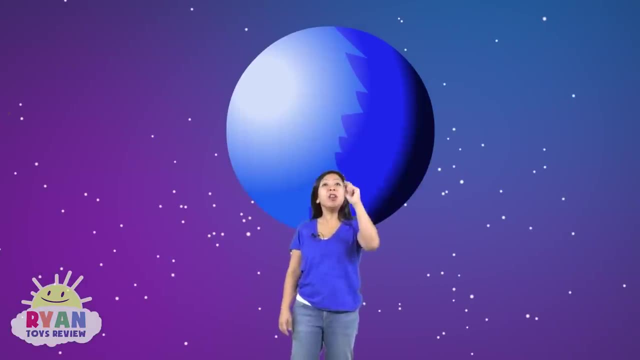 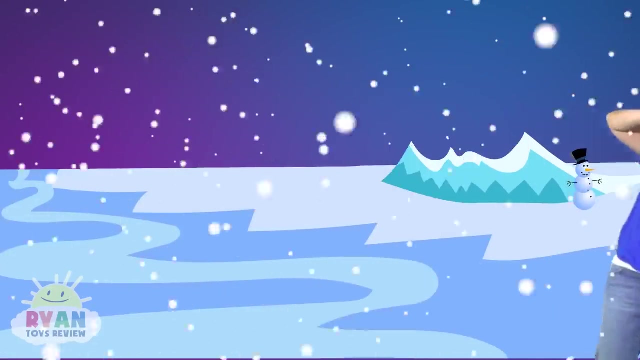 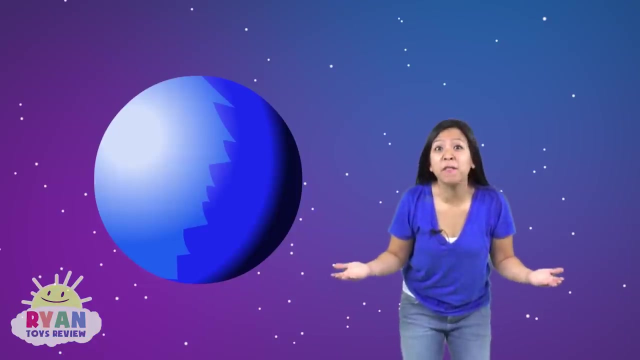 So, instead of spinning around like this, it spins around like this. And this last planet here, number eight, is Neptune. And guess what? It's really windy, Whoa, Ooh, Icy and very, very blue, because it has methane gas. 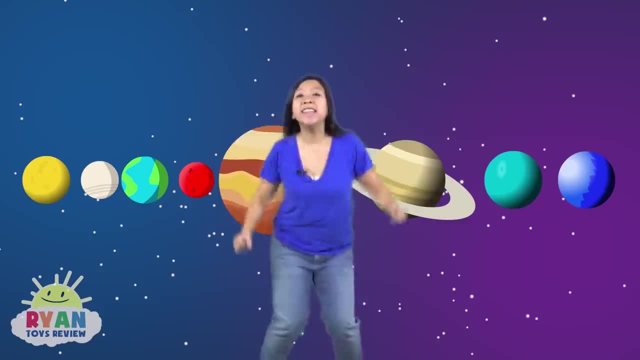 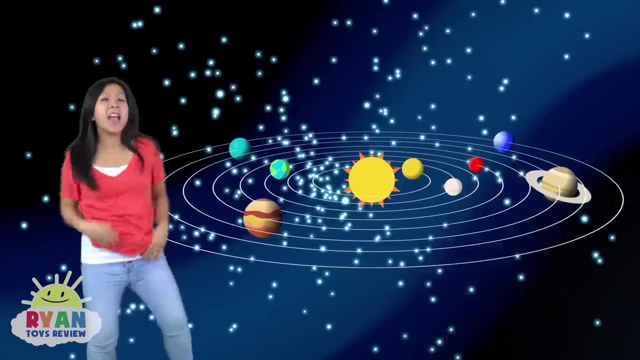 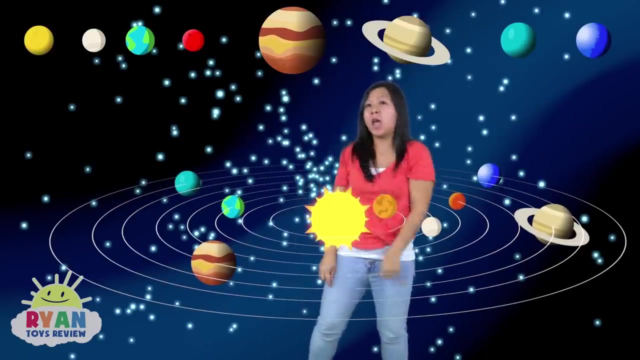 Yay, Now that we know all about our planets in the solar system, let's sing along with me. This is the planet song. If you know the order, sing along. Planets revolve around the sun. Mercury is number one. 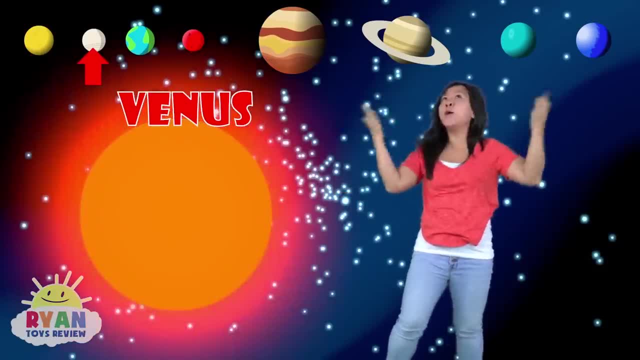 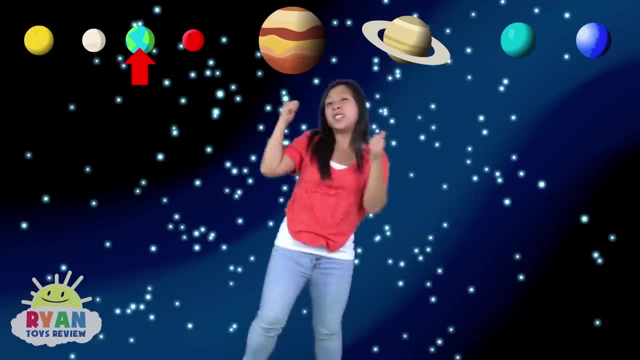 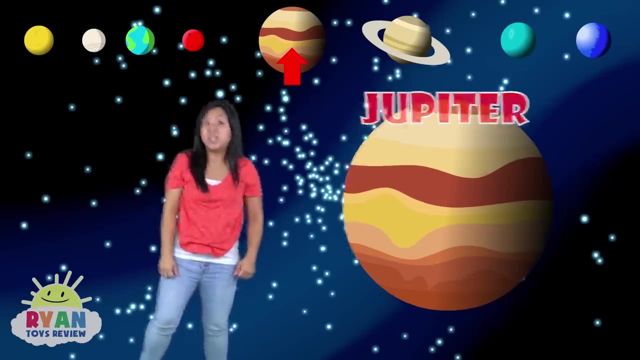 Venus is number two. It's too hot for me and you. Earth is the place to be. It's planet number three. Now let's learn some more. Mars is red and it's number four. Jupiter is number five And it's known for its giant size. 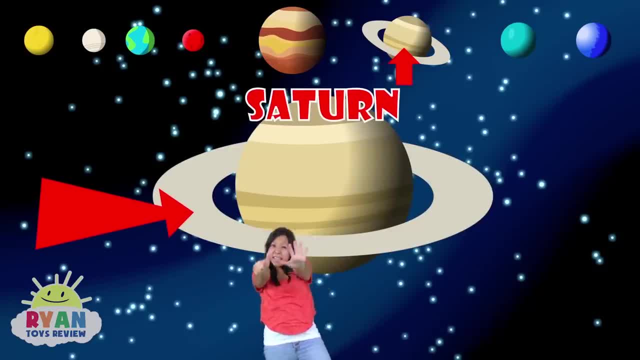 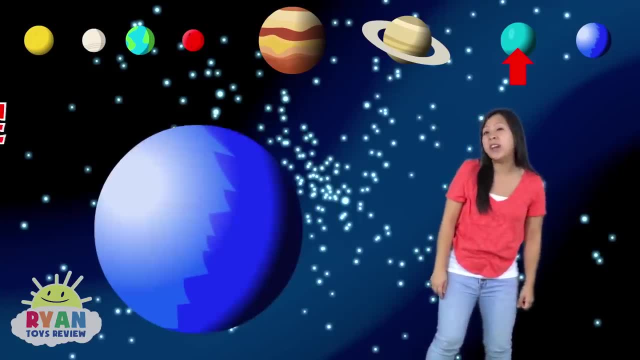 Saturn is the one with rings. It's number six in the order of things. Seven is the planet with ice. It's Uranus and it's been on its side. Number eights call Neptune. It's the last one and it's blue. This is the planet song. 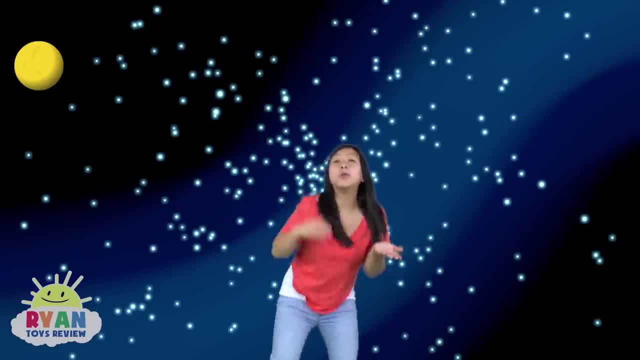 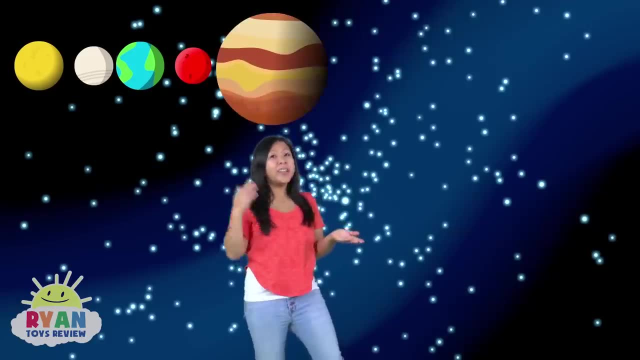 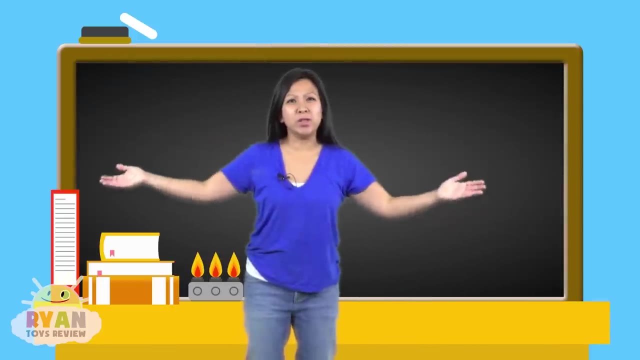 Now you know the order. sing along: Mercury, Venus, Earth, Mars, Jupiter, Saturn, Uranus and Neptune. Mercury, Venus, Earth, Mars, Jupiter, Saturn, Uranus and Neptune. Now let's do a pop quiz. Question number one: 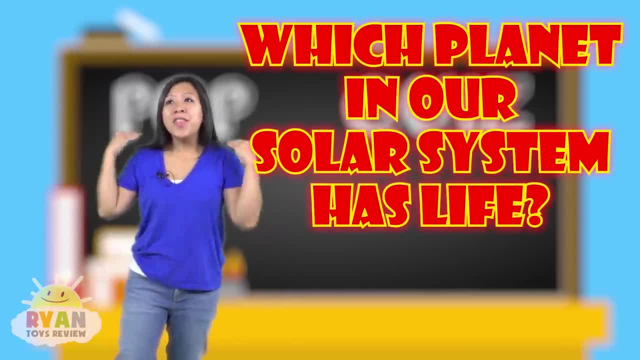 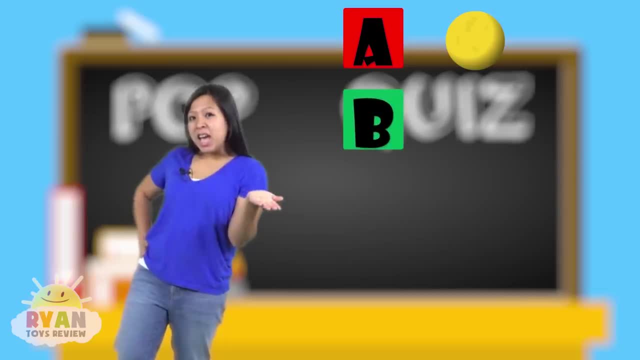 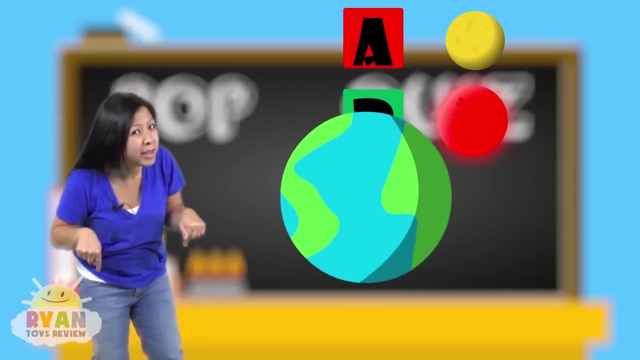 Which planet in our solar system that has life that we know of so far? A- Is it Mercury? B- Is it Mars? C- Is it Earth, the planet we're living on right now, Or is it D, Jupiter, the biggest planet? 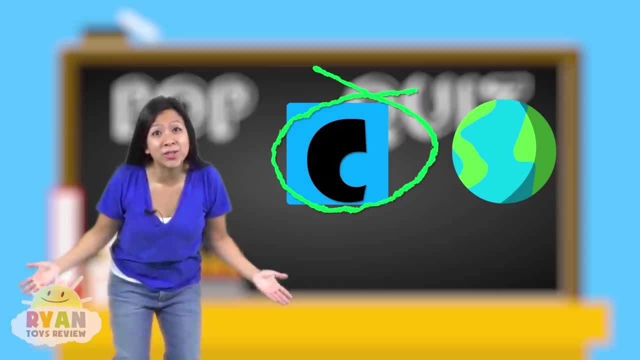 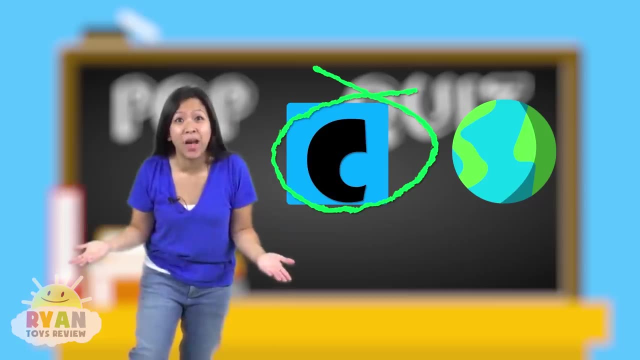 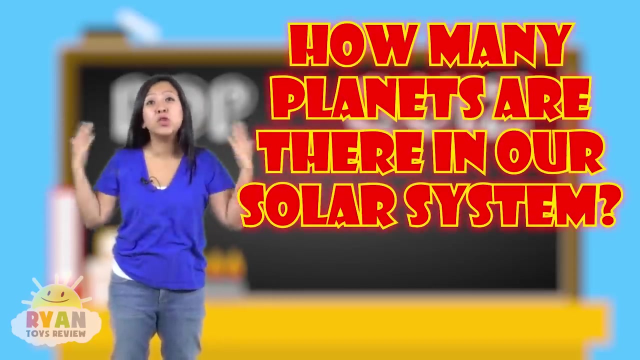 The answer is C, Earth. Did you get it right? Yay, Earth is the only planet that we know of right now that has life. How cool is that right? Question number two: How many planets are there in our solar system? A, Is it 60?? B Is it 870?? C- Is it 8?? Which one? And the answer is C: 8!. There's 8 planets in our solar system. Let's quickly name them again: There's Mercury, There's Venus And then there's Earth. 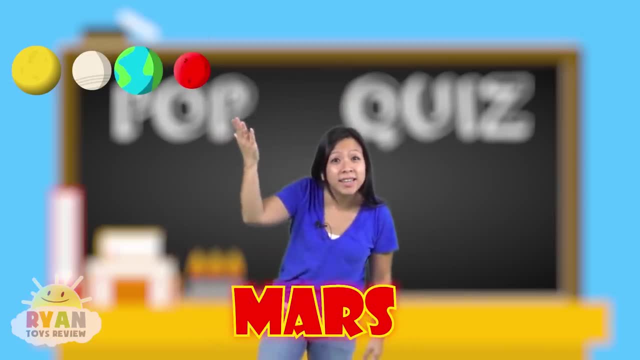 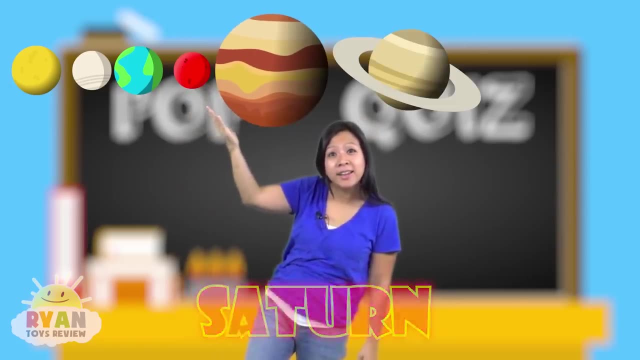 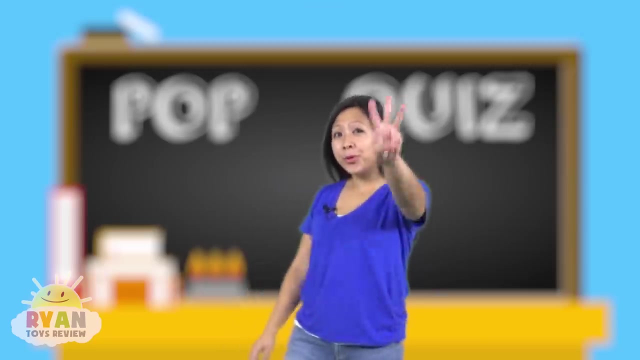 There's Mars, Jupiter- Super big Saturn, Uranus And Neptune. Did you get it? Last question, number three: Which planet in our solar system that has life that we know of so far? Which planet in our solar system is the biggest? Do you remember? 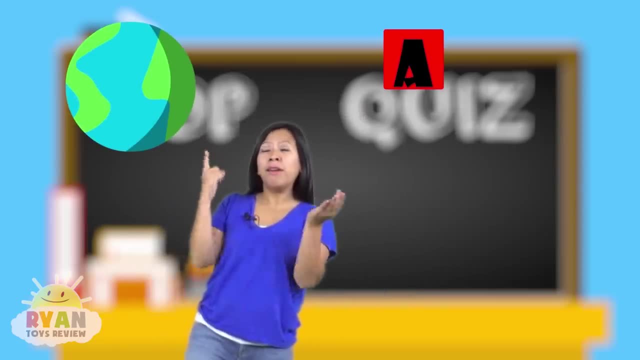 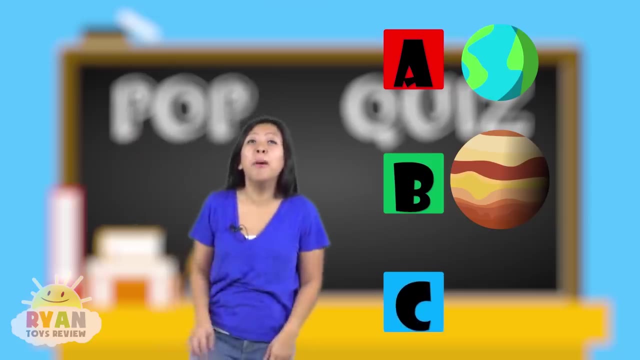 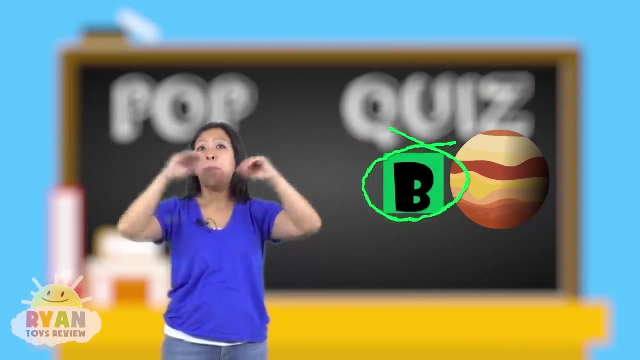 Is it A- Earth, Is it B- Jupiter Or is it C- The moon? And the answer is B Jupiter. It's the biggest planet in our solar system. Look how big it is. Don't come any closer- So huge. 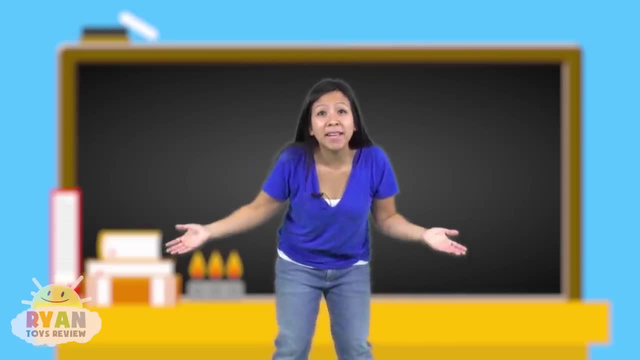 Wow, Good job. Good job answering the pop quiz, And if you didn't get it right, just try again next time. Now that we know all about our planets, let's go back and tell Ryan: okay, Let's go. Wow. 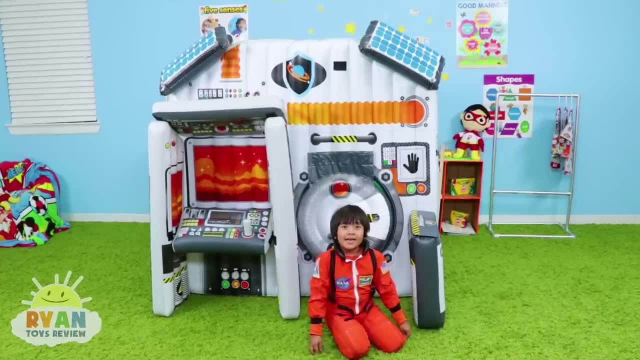 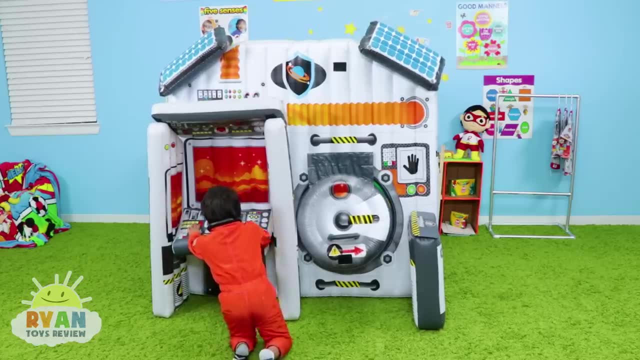 Okay, guys, I'm going to go to planet Mars to find mommy. Where did she go? It's set to Mars. There we go. Okay, guys, I'm going to go to planet Mars to find mommy, Where did she go? It's set to Mars. 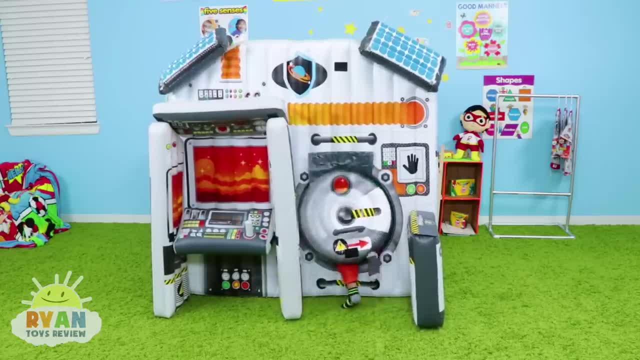 Okay, guys, I'm going to go to planet Mars to find mommy. Where did she go? It's set to Mars. There we go, Bye, Okay. 3,, 2,, 1.. So those are all the planets in our solar system. 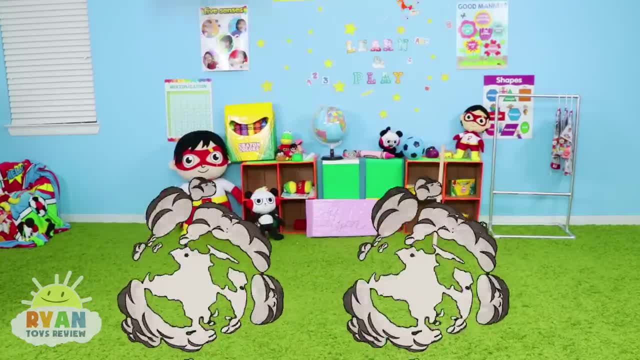 Wait, Ryan, Where did he go? Did he go to outer space without me? You can get your own Ryan's World toys and clothing at Walmart and Walmartcom. They're free and you can buy them at the store. I'll be right back.